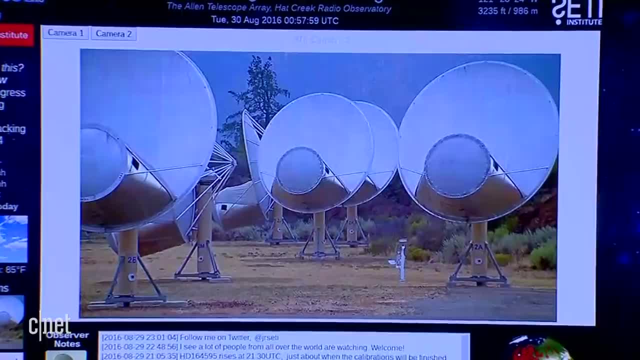 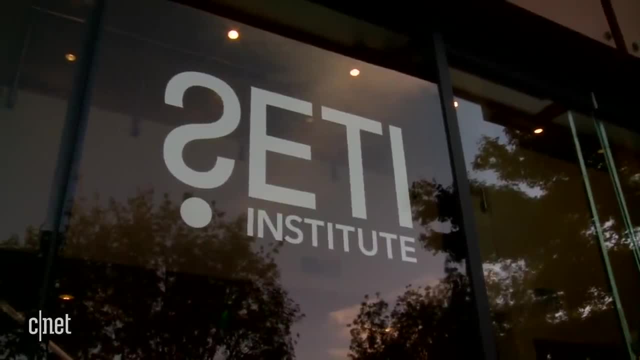 signs of life on other planets, but after just one year Congress pulled funding. But that search hasn't stopped. One of the main groups pushing it forward is the SETI Institute, which gets partial funding from NASA and has a team of scientists studying exoplanets. 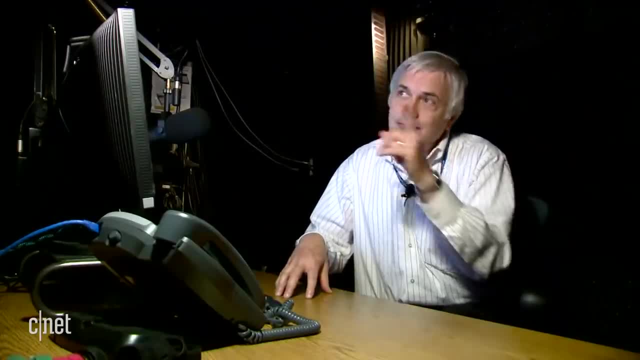 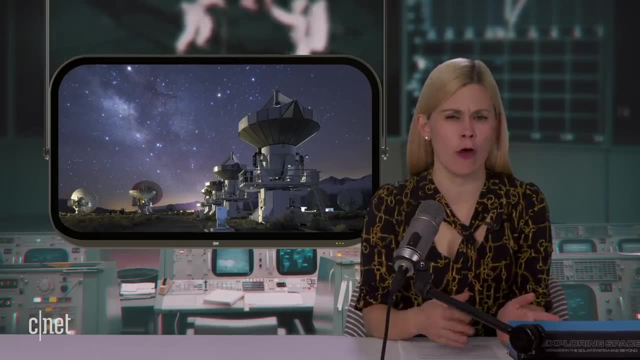 examining how planets were formed and and researching the astrobiology needed to support life on other worlds. I know what you're thinking: The hunt for alien life is real, but we're not overrun with little green men What gives? Well, there's no need to go full Area 51 on me. 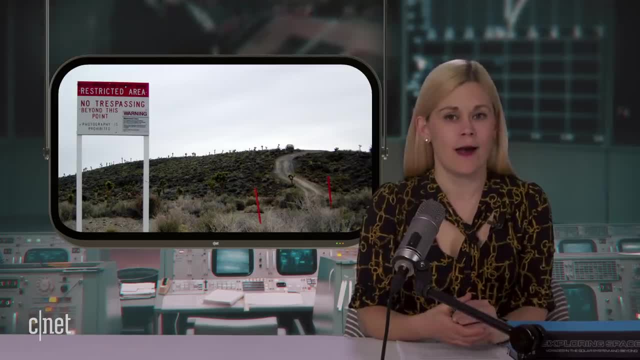 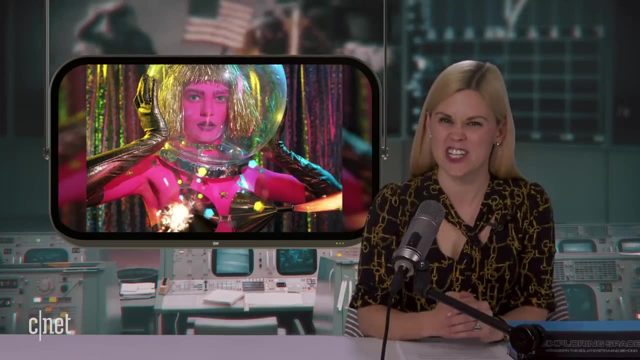 No, that's some 41. Why does this keep happening? The reason we haven't become an alien ant farm is because, despite all those party city costumes you've bought, alien life isn't actually that sexy. Let's take a journey through our search for extraterrestrial intelligence. 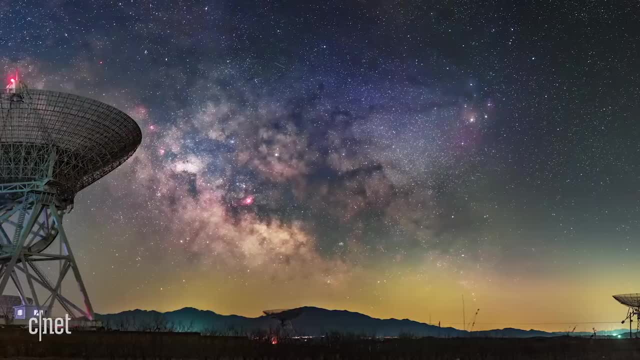 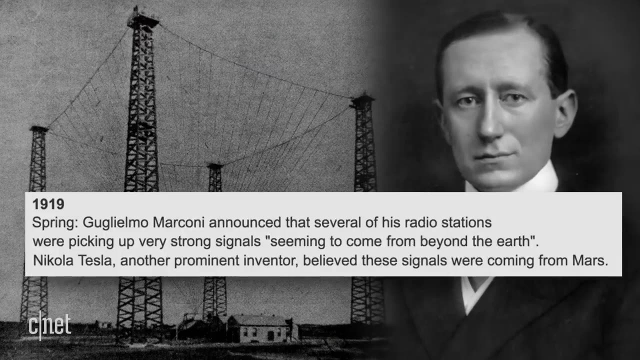 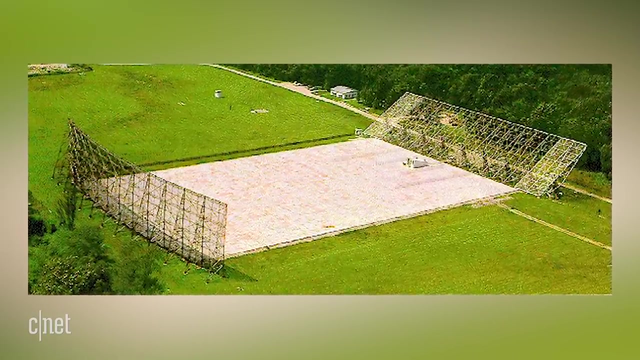 and all the ways that scientists have made it boring. First up there's radio astronomy. We've been studying radio signals for signs of life ever since Marconi supposedly picked up transmissions from beyond Earth back in 1919. But one of the biggest discoveries came in 1977 from the Big Ear radio telescope in Ohio. 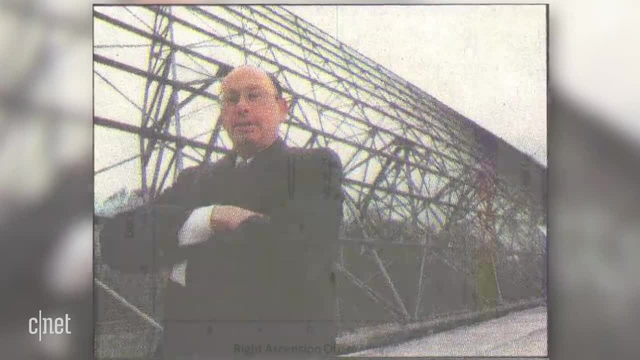 Astronomer Jerry Ehman was picking through data from the Big Ear- No, that's not a gross way, I'm not saying he was using a Q-tip- And in that data he found a radio signal that lasted roughly one minute. 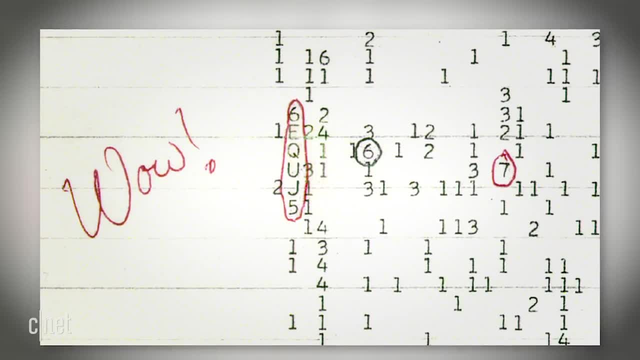 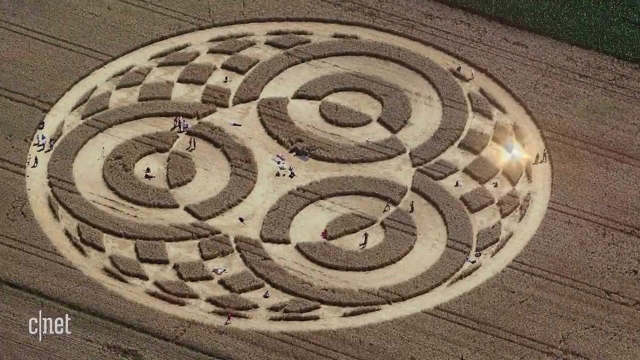 He wrote the word WOW on the printout because apparently he's a kid in a 1950s comic book, and it's been known as the WOW signal ever since. While this discovery sounds cool, it wasn't exactly some secret alien message. 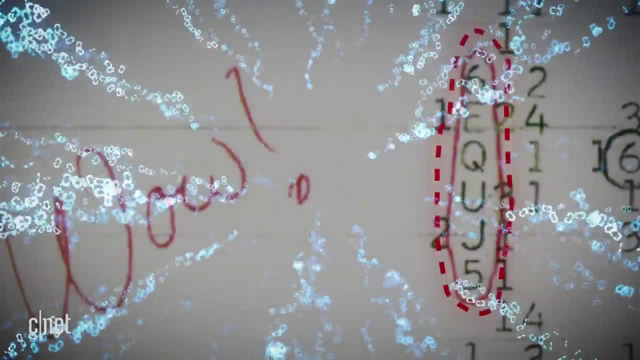 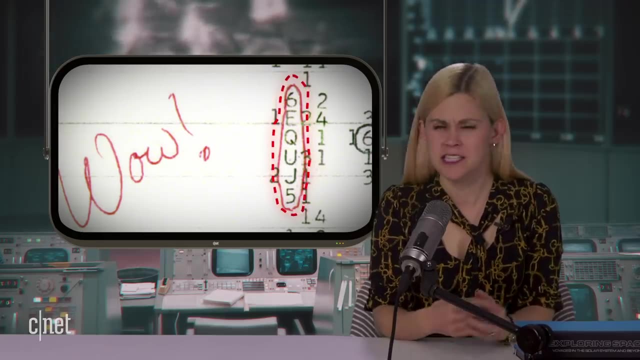 It was just a mash of encoded data represented by six characters: 6-E-Q-U-J-5.. Secugious, Secugious. Yeah, it's effectively just an intercalation and it's not a galactic vanity. license plate. 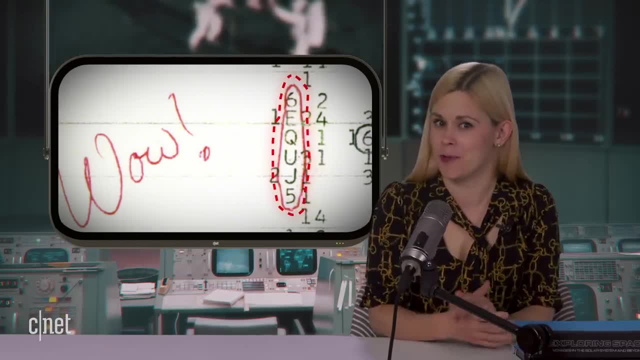 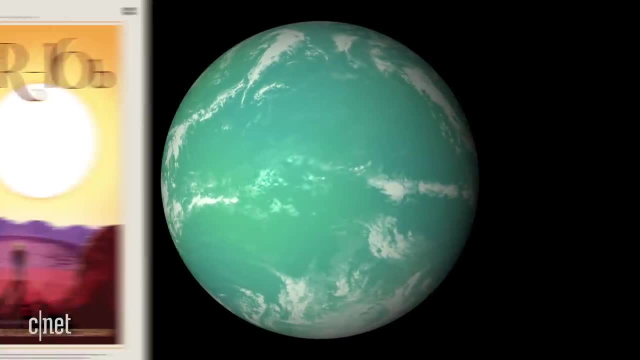 See kids, Science can be boring. Next up, exoplanets. Hey, cool Planets just like Earth with the perfect conditions for life. Hell, these things even have their own NASA posters. Surely we'll find aliens there, right? 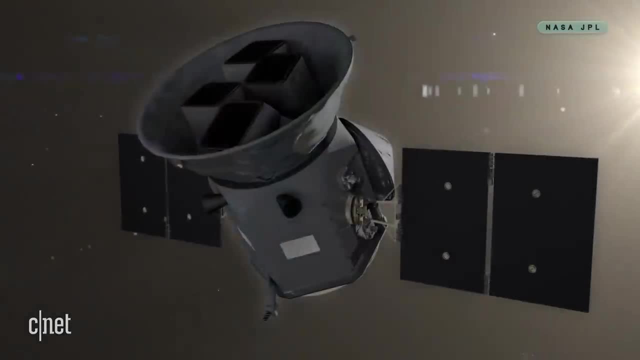 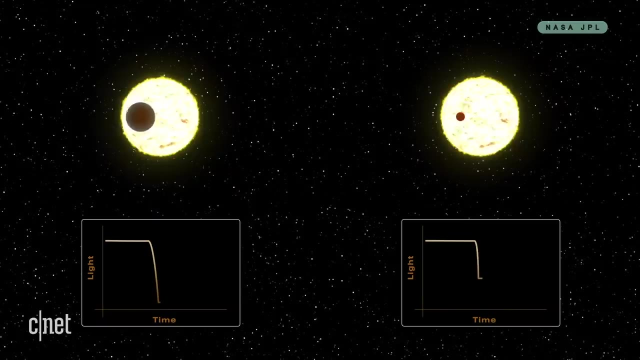 Well, Right now we search for exoplanets using instruments like TESS, the Transiting Exoplanet Survey Satellite. TESS finds planets by monitoring stars to see drops in their brightness caused by a planet passing in front. As far as finding planets, it's not a big deal. 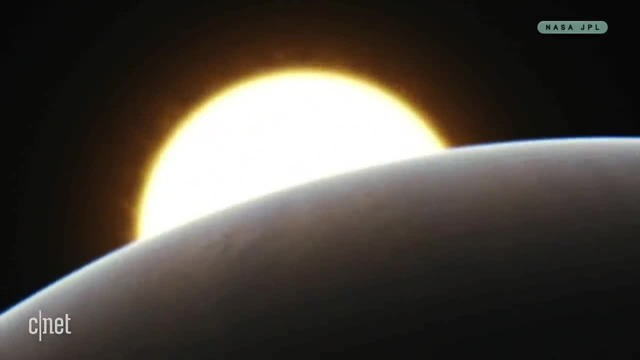 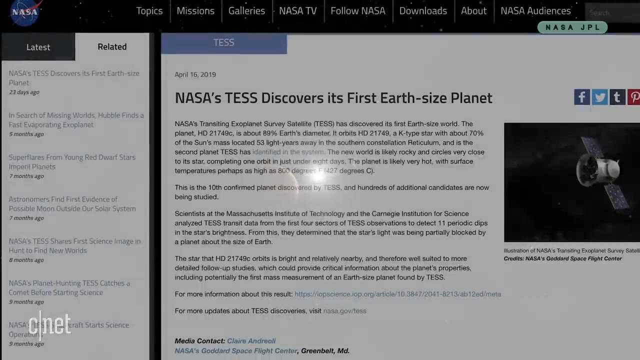 If you're just finding perfect alien planets, that's the equivalent of choosing your husband because he walked in front of the screen at the movies. Still, TESS has found more than 500 exoplanet candidates and in April 2019, it found its first Earth-sized world. 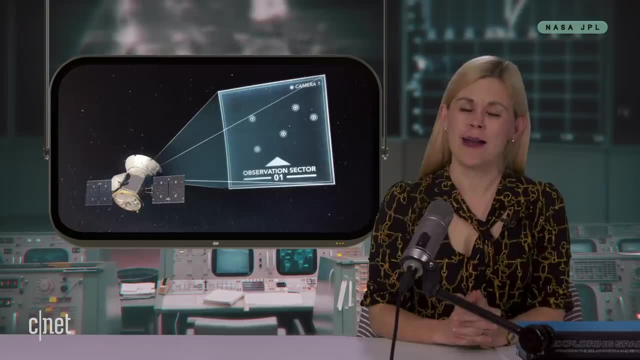 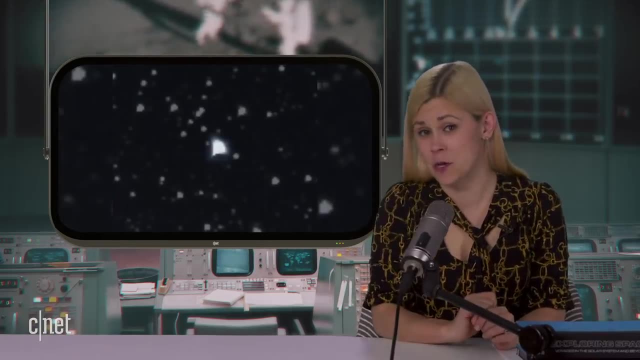 Now, that's cool Stars. They're just like us. Well, no, because while it could look like this, right now it looks like this, And that's not even the exoplanet. That's its star. Also, it's called HD 21749C. 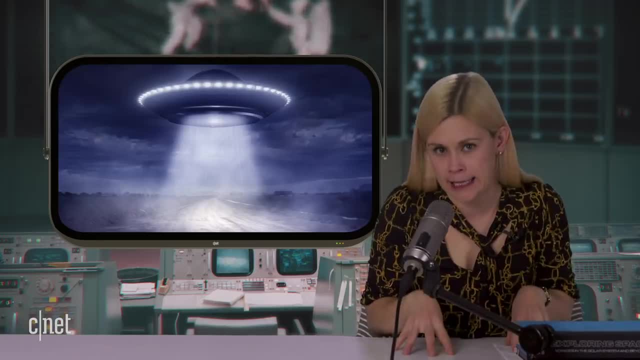 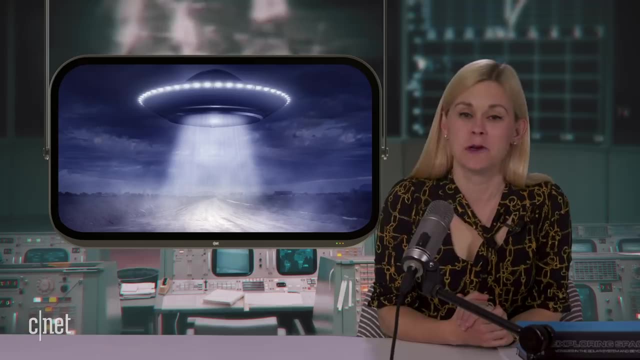 Science Boring. Okay, so this is the alien episode. Surely we have something really cool and weird that we're doing in the search for extraterrestrial intelligence. Well, you're in luck because I have some 100% real, 100% bonkers, ET factoids for you. 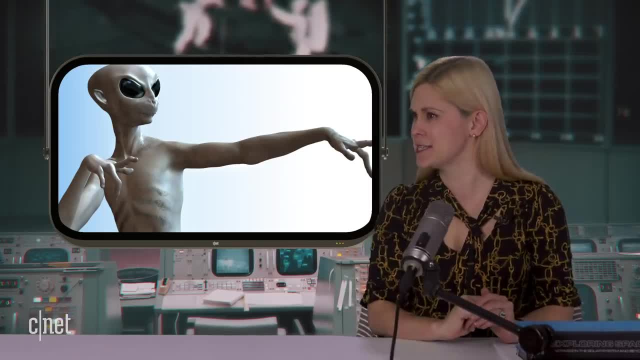 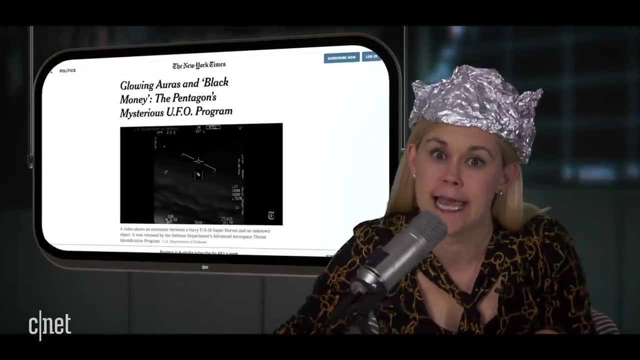 Could I get something in a YouTube conspiracy theorist filter for this next vid? Thank you. First up, let's talk about the Pentagon's secret UFO program. All right, in 2017, the New York Times reported that the Fed spent $22 million on a secret program at the Pentagon. 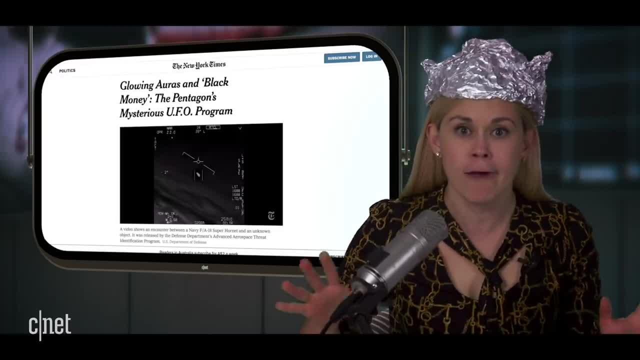 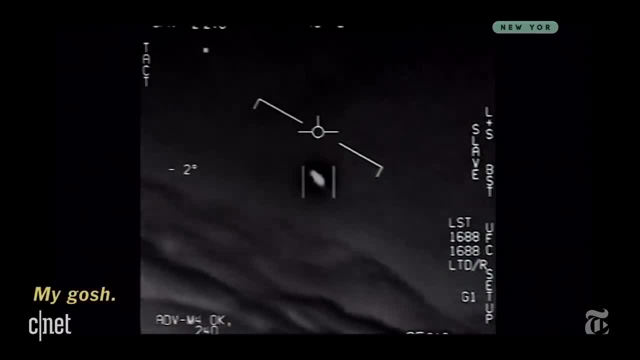 to look into reports of unidentified flying objects. Apparently, defense defunded the program in 2012,, but it might still exist. Wake up, sheeple. You want more UFOs? Good, According to a Politico report from April 2019,. 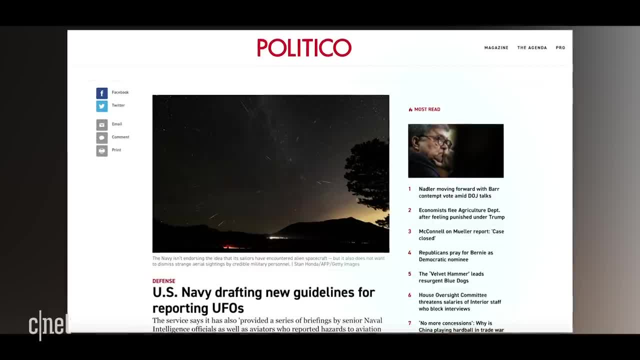 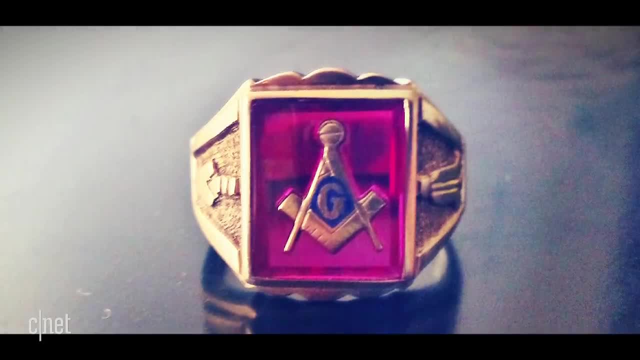 the US Navy is working on procedures to report unidentified aircraft, so quote incursions can be made to the quote authorities, which we all know is code, for the Freemasons are building a secret UFO database And finally adjust your hearing membranes- lizard people. 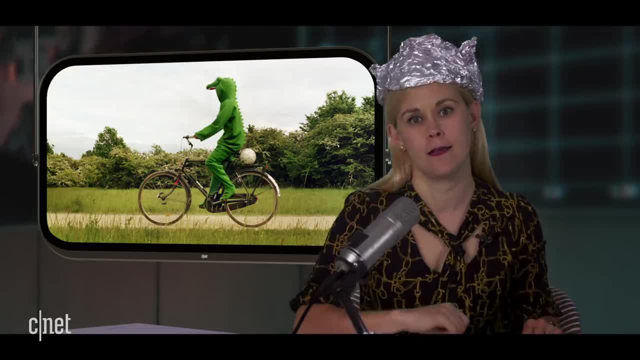 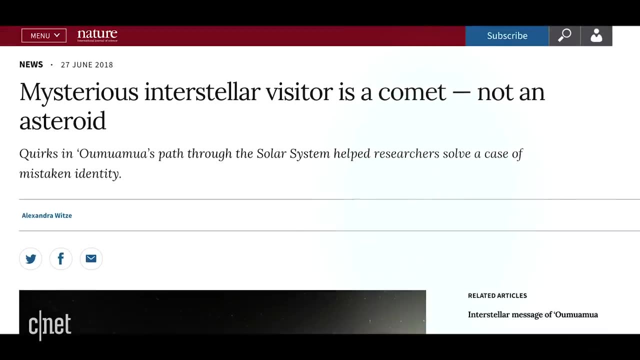 because it turns out, we were the aliens all along. Remember back in 2017, when the Oumuamua asteroid floated into our lives? We now know it's an icy comet, but back then Harvard scientists thought it could be a quote. 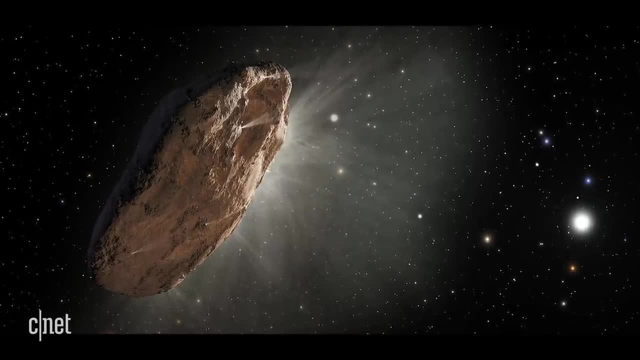 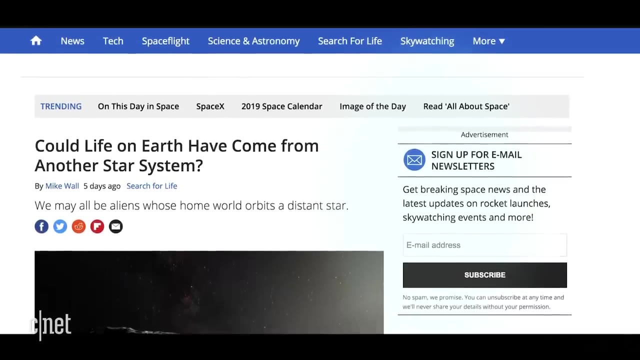 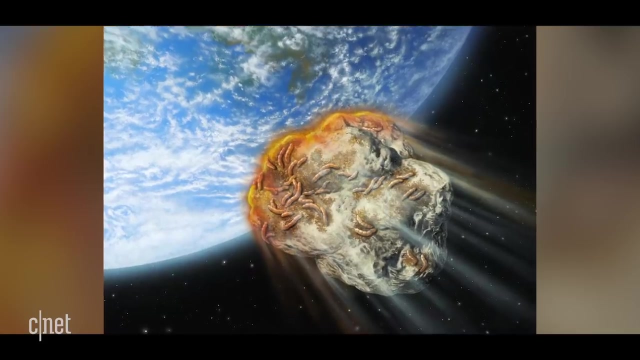 fully operational probe sent intentionally to Earth's vicinity by an alien civilization. Not only that, but some scientists believe interstellar objects like Oumuamua could provide enough insulation and radiation protection to preserve living organisms on an interstellar journey. It's a process called panspermia.